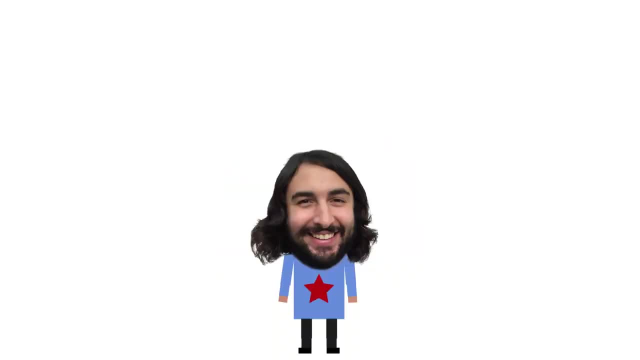 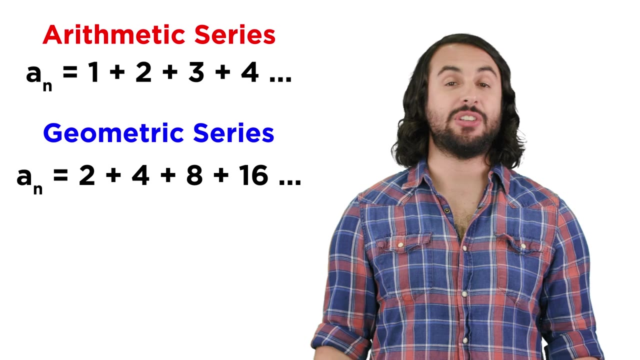 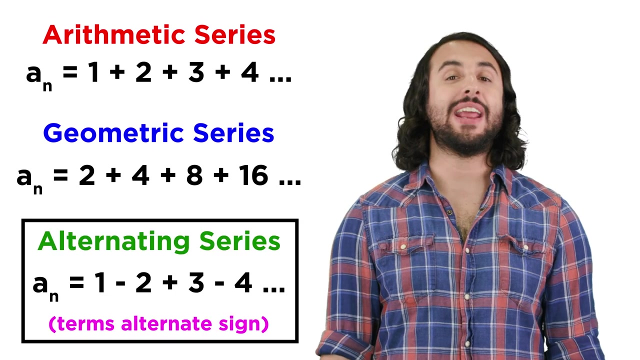 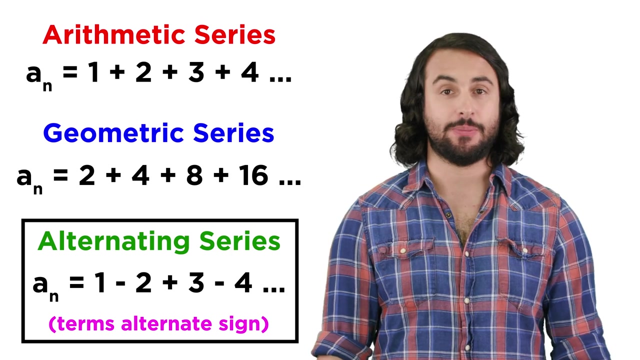 It's Professor Dave. let's look at alternating series. We've examined arithmetic sequences and geometric series, so let's look at another type of series now. An alternating series is one in which the signs of the terms in the series alternate between positive and negative values. 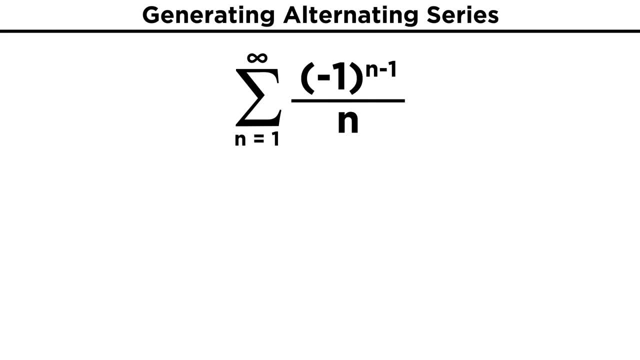 How can we produce a series like this? In order to produce an alternating series, there will usually be a term involved whereby the number negative one is raised to some exponent like N or some term with N in it. For example, take the series negative one to the N minus one power over N from one. 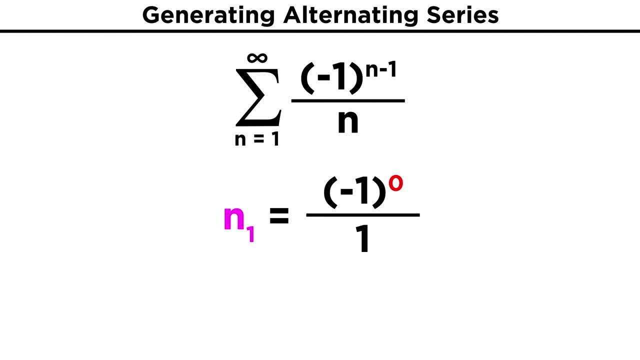 to infinity. For the first term we are raising negative one to the zero power, which is one, and then we divide by one, so we just get one. But then for the second term, negative one is raised to the first power, so we leave. 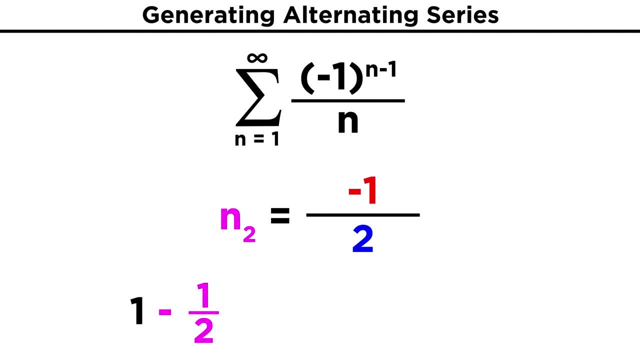 the negative one divide by two and we get minus one half. For the third term, the negative one is squared to give positive one and we get one third. If we continue in this manner, we see how the number in the denominator increases by. 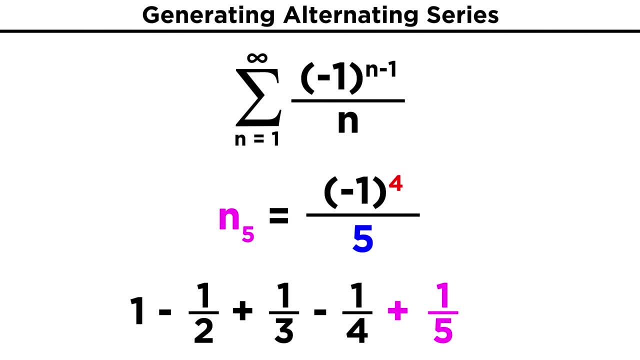 one each time, as expected. but because the term in the numerator alternates between the positive and negative one, the terms in the series alternate between positive and negative all the way to infinity. So any time you see a series and there is a negative one in parentheses being raised, 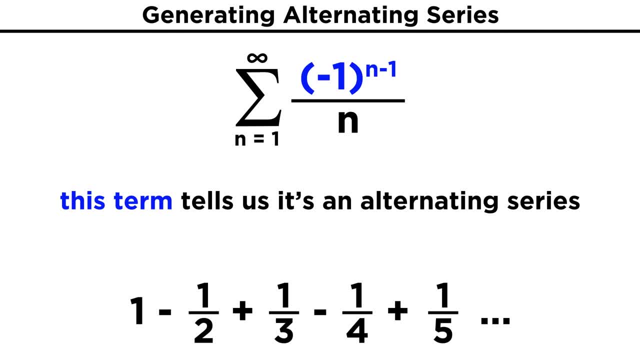 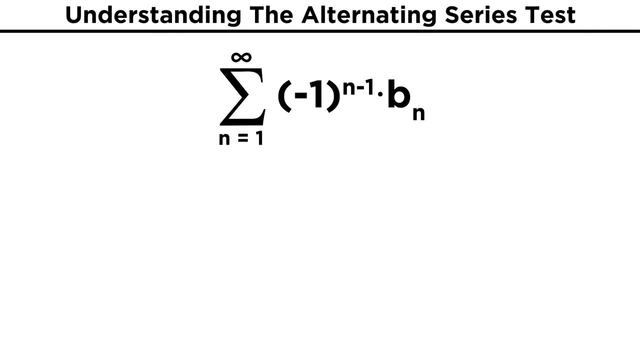 to the N power or something similar. you know that you are looking at an alternating series. Because of these alternating signs it becomes trickier to assess whether the series will converge or diverge, But we can use something called the alternating series test. 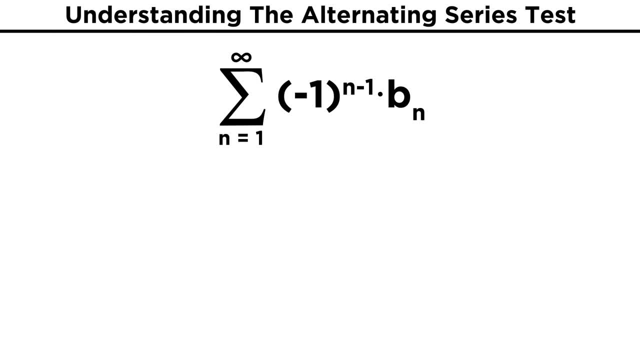 This test says the following: Let's say we have some series in the form of negative one to the N minus one times B sub N, which gives us B one minus B two plus B three minus B four and so forth, where B sub N is greater than zero. 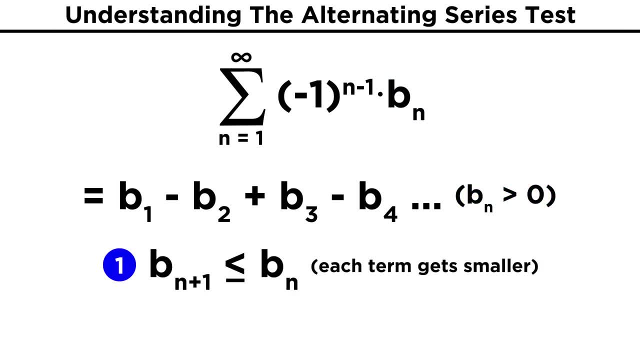 If B sub N plus one is less than or equal to B sub N, or in other words, if each term in the series is smaller than the last disregarding sign, and also if the sequence B sub N goes to zero in the limit of infinity, then the alternating series will be convergent. 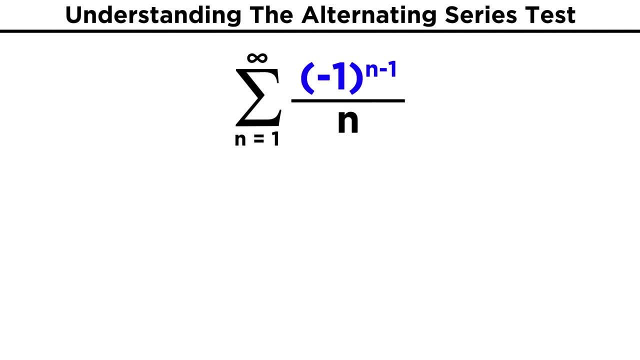 So, for example, with that first series we looked at, we can pull the term in the numerator to the side and B sub N is therefore represented by one over N. Each term in this series is smaller than the previous And in the limit of infinity one over N goes to zero. so both criteria are met and this 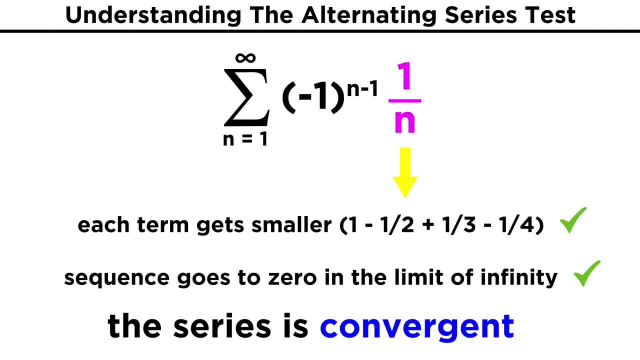 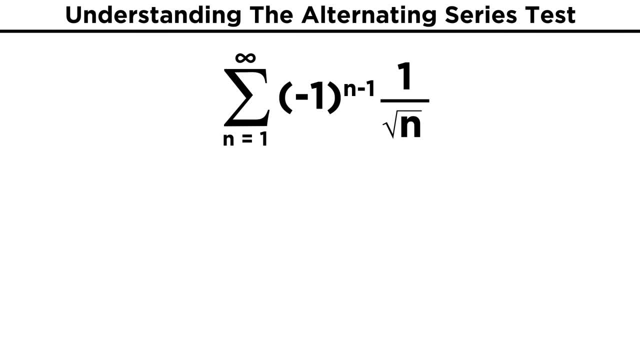 is indeed a convergent series. Let's apply this to a few series to make sure this sinks in. Take this one that is the same as our previous example, except with root N in the denominator. Does each term in this series get smaller? 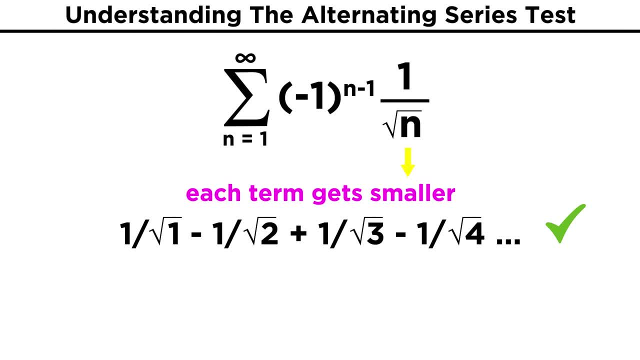 As N increases, its square root increases. So the fraction gets smaller as we go And in the limit of infinity, this term does become zero. Both criteria are met and this sequence converges. What about this? one negative one to the N times the quantity three, N minus one over. 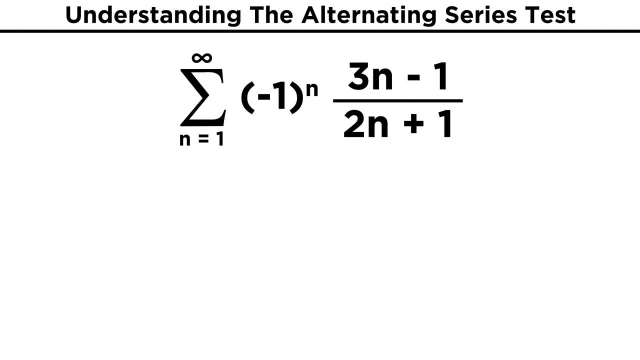 the quantity two, N plus one. Here does each term get smaller. Well, we have a larger multiple of N on top. As N gets very large, the plus and minus one get smaller. Well, we have a larger multiple of N on top. As N gets very large, the plus and minus one get smaller. 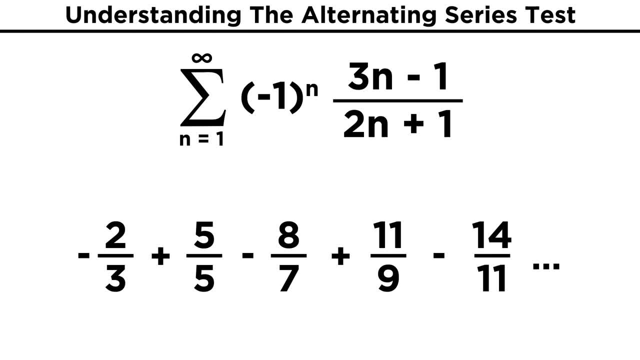 Well, we have a larger multiple of N on top. Well, we have a larger multiple of N on top. All the plus and minus one terms will be negligible, and we just have the numerator getting increasingly larger than the denominator. The terms are therefore not getting smaller, and in this case that means that the series 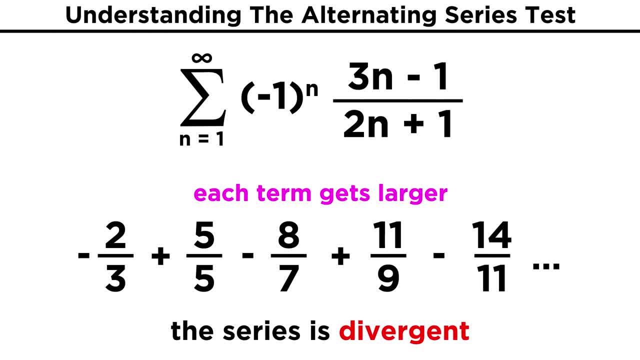 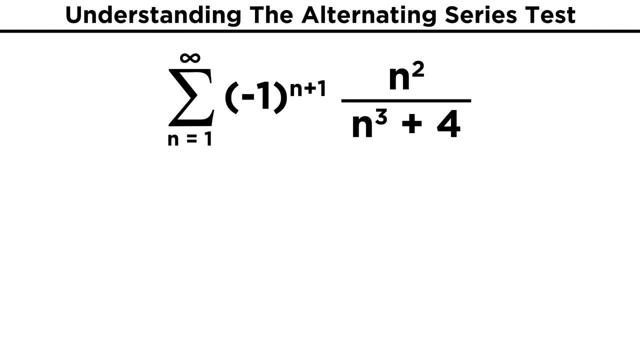 is divergent. How about this one with negative one to the N plus one times N, squared over the quantity N cubed plus four? As we might have realized by now, the slight discrepancies in the equation would be much. the exponent associated with negative one are not really relevant. so let's look at. 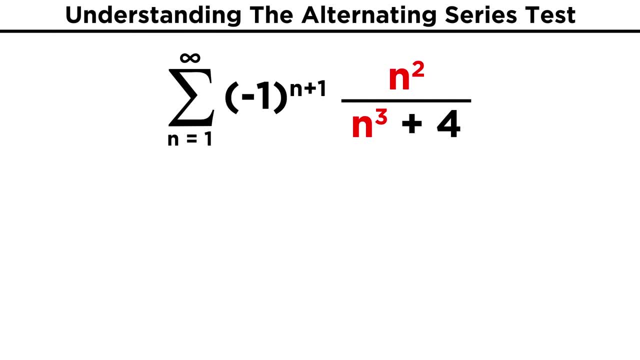 the rest, With a higher power of n in the denominator, we can be sure that each term in the series is getting smaller. Does it go to zero in the limit of infinity? Well, just plugging in infinity, we get infinity over infinity. so let's divide top and bottom. 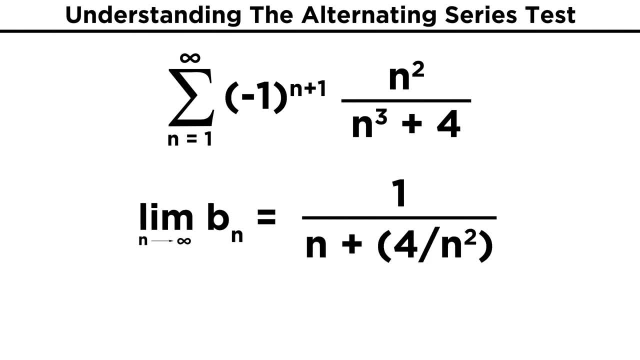 by n squared, That gives us one over the quantity n plus four over n squared. Now, plugging in infinity, we get one over the quantity, infinity plus zero, or one over infinity, which is zero. Both criteria are met and this series converges. 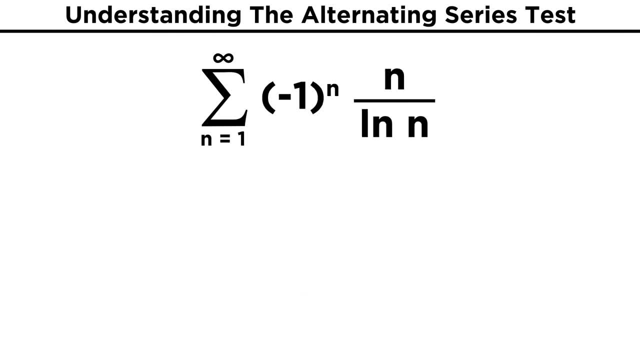 Let's do just one more negative one to the n times n over the natural log of n. Let's do just one more negative one to the n times n over the natural log of n. Do the terms increase or decrease? Well, the natural log of n will always be smaller than n and it will increase at a slower rate. 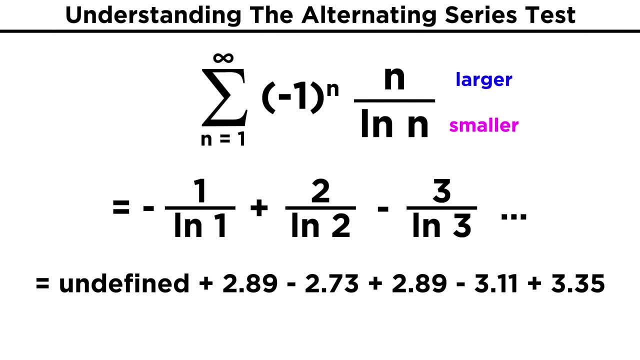 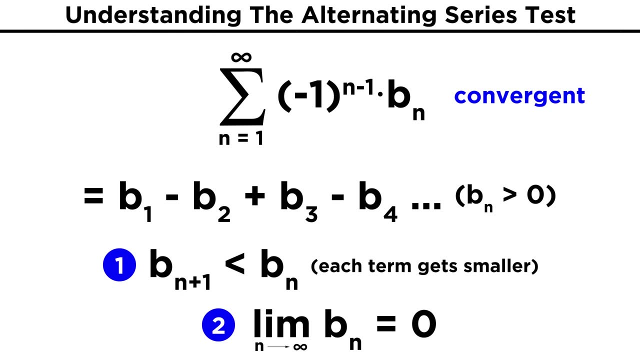 than n does, as we can see by plugging in a few values for n. so the terms are increasing and this series is divergent. So now we know how to look at alternating series and test for convergence, but we must now describe two different types of convergence. 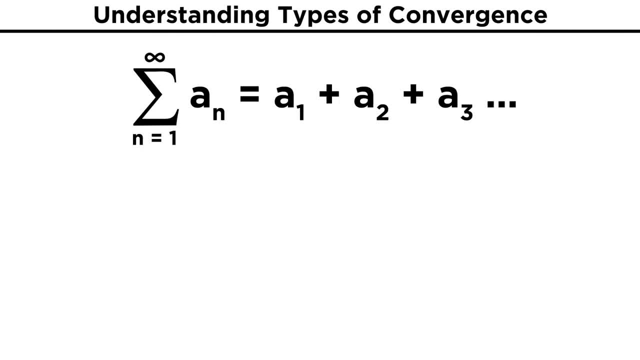 Let's say we have some series, A sub n, from one to infinity. Now let's take the absolute value of that series, which means we are taking the absolute value of every term in that series. If A sub n is convergent and the absolute value of A sub n is also convergent, then 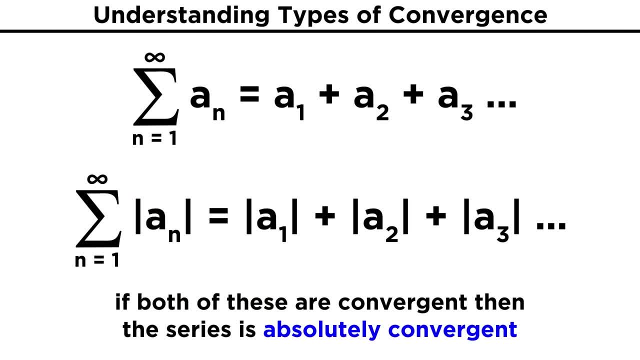 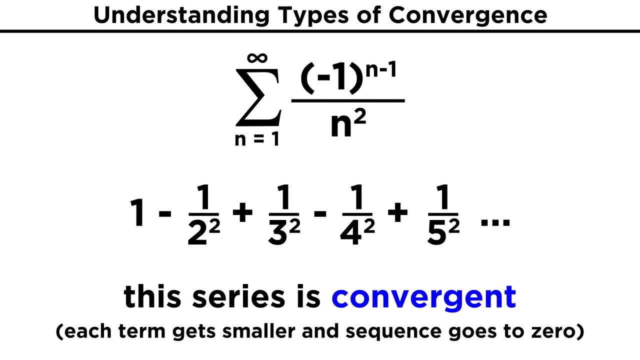 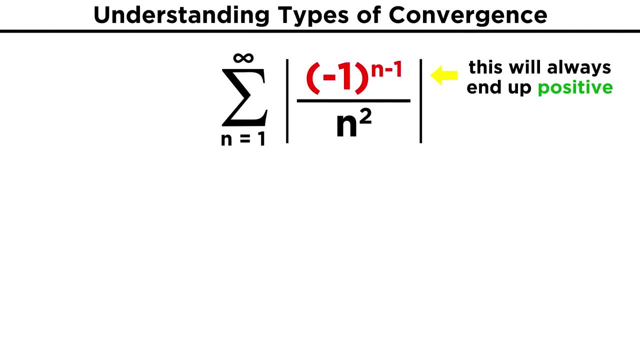 that series is called absolutely convergent. OK, so Take number two. alright, Take sentences. Very well, Thank you very much. You're welcome. minus one over N squared. we said that this series was convergent. Now let's take the absolute value of this series. 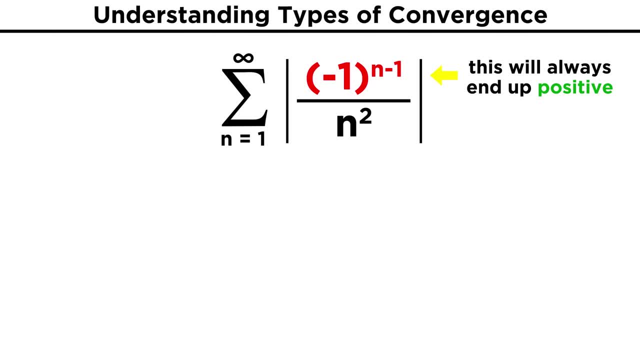 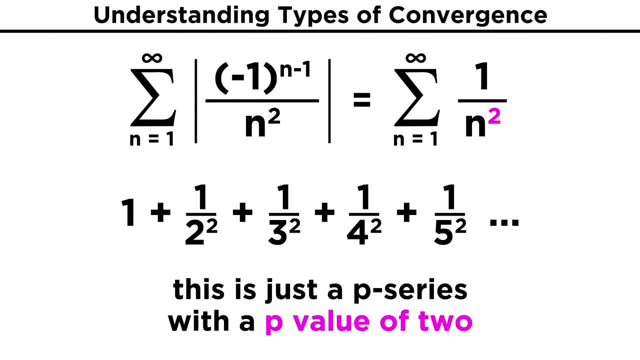 This means that whenever the negative one gives us a negative value for a particular term in the series, we just make it positive instead. So rather than an alternating series, we just get a regular P series with a P value of two, as though the negative one term was not present. 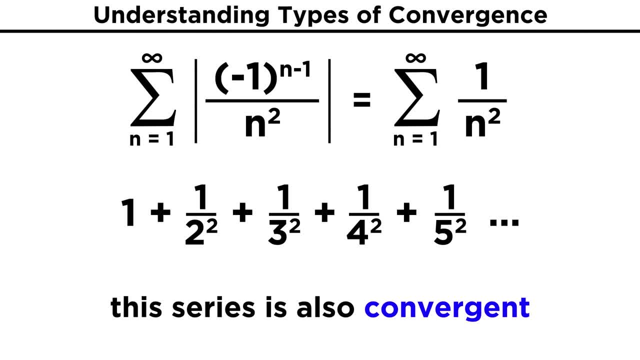 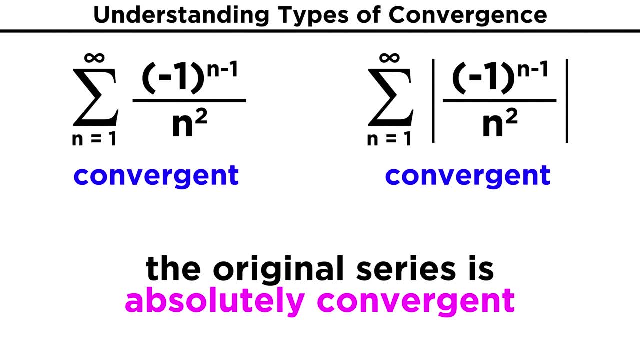 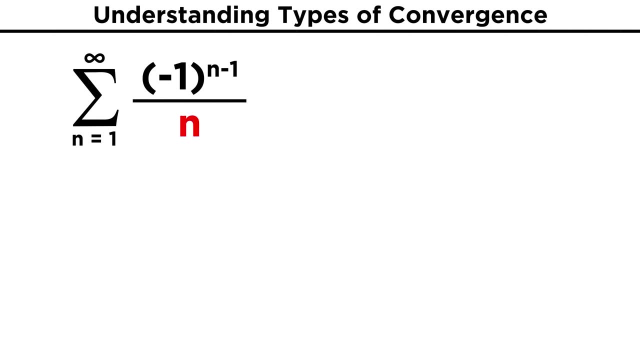 We know that this series is also convergent for reasons discussed in the previous tutorial. Since they are both convergent, then the original series is absolutely convergent. On the other hand, let's modify this slightly and take away the exponent in the denominator. 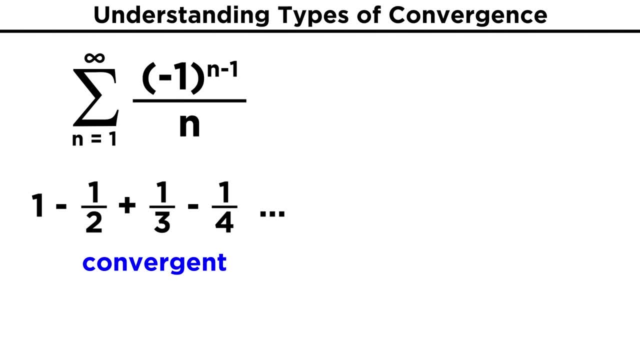 leaving simply N. That will give us a different alternating series which we know is also convergent. However, when we take the absolute value of this series, which turns all the terms positive, we get another P series, but this time with a P value of one. 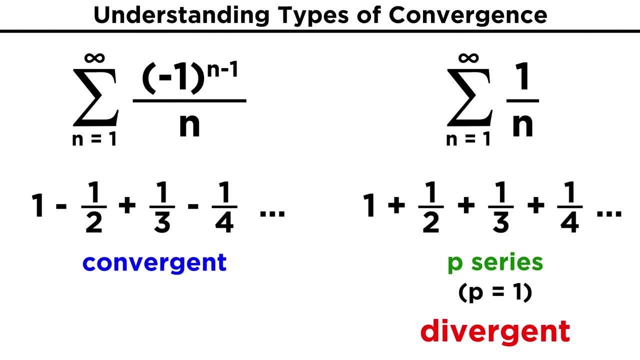 Any P series with a P value of one or less will be divergent, and so we say that the original series is conditionally convergent. This is different from being absolutely convergent, because taking its absolute value produces a series that is divergent. 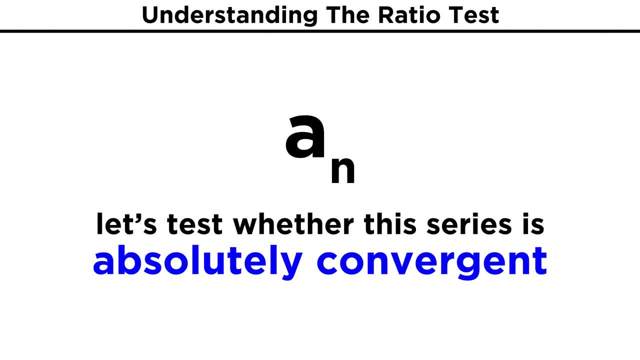 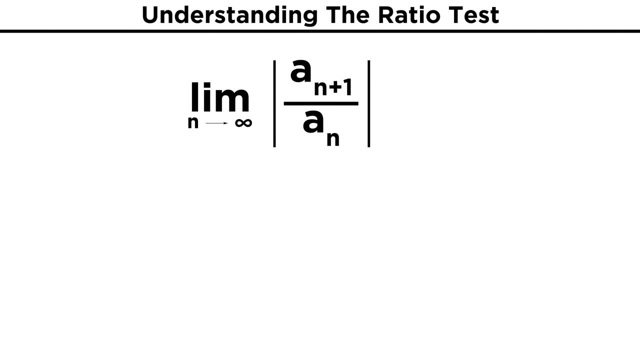 There is a test that is helpful in determining whether a series is absolutely convergent, and it is called the ratio test. We can place A sub N plus one over A sub N to form a ratio and take the absolute value. Then we take the limit of this ratio as N approaches infinity. 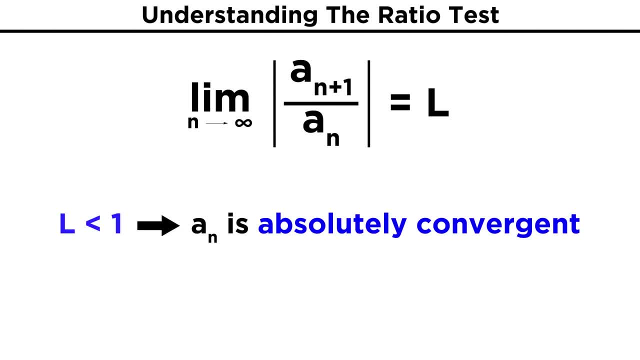 This limit will equal L. If L is less than one, then we can take the absolute value of the ratio as N approaches infinity. If L is less than one, then we can take the absolute value of the ratio as N approaches infinity. If L is greater than one, then the series A sub N is absolutely convergent. 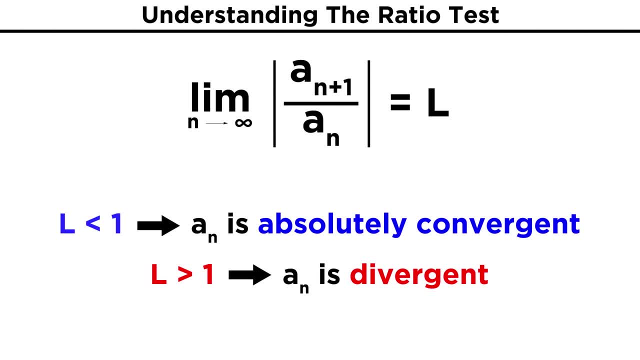 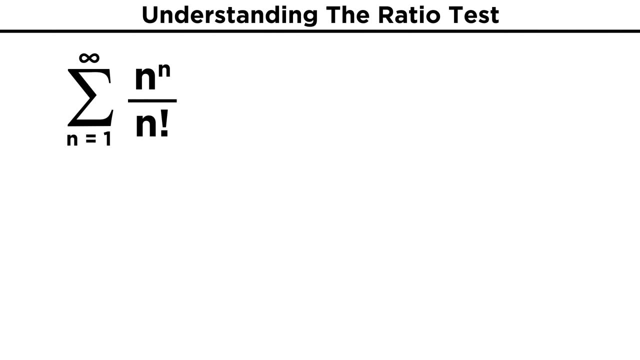 If L is greater than one, the series is divergent, And if the limit equals one, the ratio test is not useful and it can't tell us any information about the series. Let's try one example that requires this ratio test. How about the series N to the N power over N factorial? 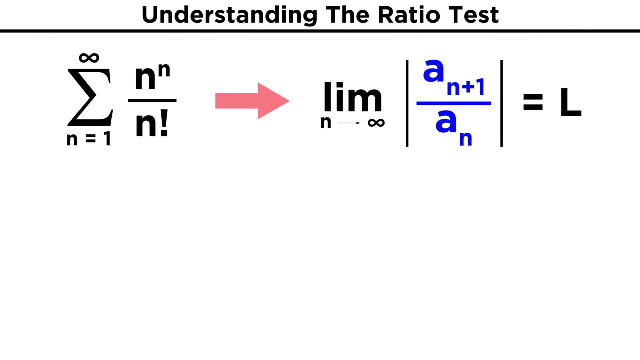 We need to get the ratio of A sub N plus one over N factorial. So we divide by a fraction and we get the ratio as N plus one over A sub N. For A sub N plus one, we just put N plus one wherever N was, so we get the quantity N plus. 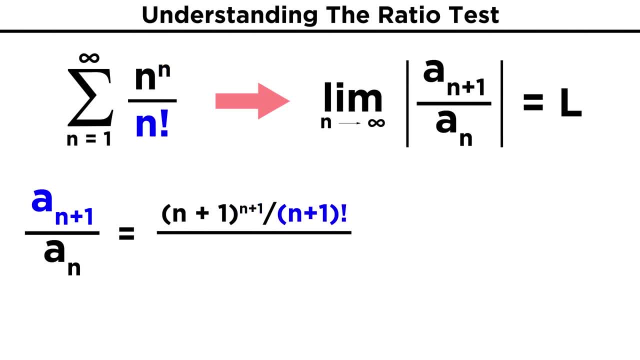 one raised to the N plus one power over N plus one factorial. Then we divide that by the original series, N to the N over N factorial and we take the absolute value of all that. But everything is positive. so the brackets just go away. 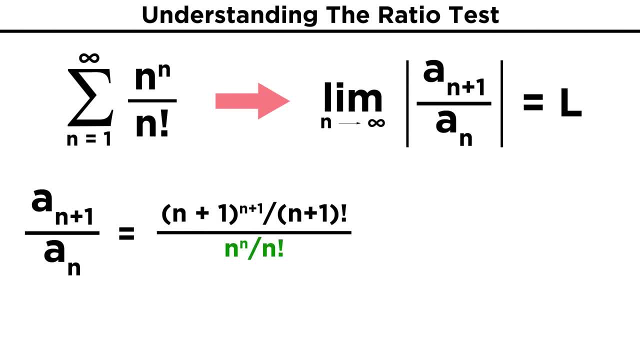 We can now divide by a fraction. Now, dividing by a fraction is the same as dividing by a fraction. But I don't want to divide by a fraction same as multiplying by its reciprocal. so let's flip this denominator and bring it up here. 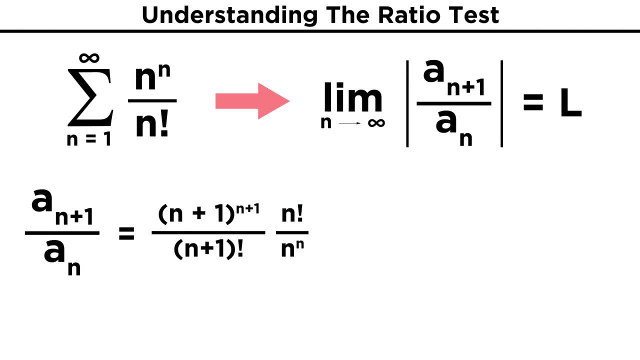 Looking at all this, we should be able to cancel some things if we get clever. For one thing, we have n plus one factorial as well as n factorial. Well, we know that n plus one factorial will be n plus one times n times n minus one. 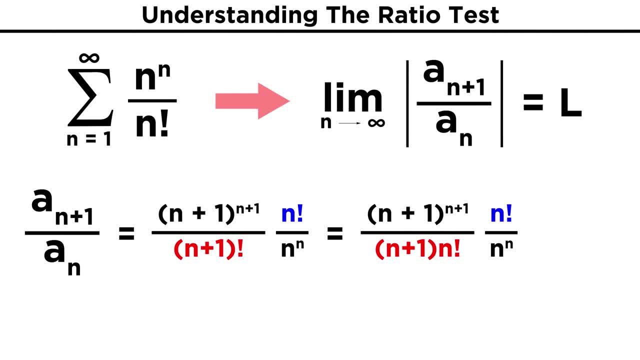 and so forth. So really we can just say that this is equal to n plus one times n factorial, since the rest of this is just n factorial anyway. Then on the top, raising this binomial to the n plus one power is the same as n plus. 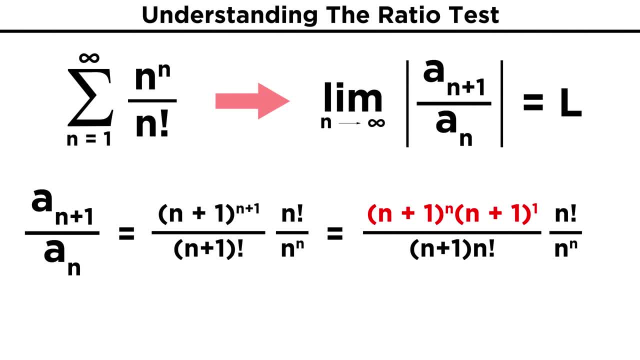 one to the n power times, n plus one to the first power. This is just using a property of exponents in reverse. Now things look pretty good. We can cancel out an n plus one from top and bottom, And we can do the same with n factorial, leaving us with n plus one to the n power over n to 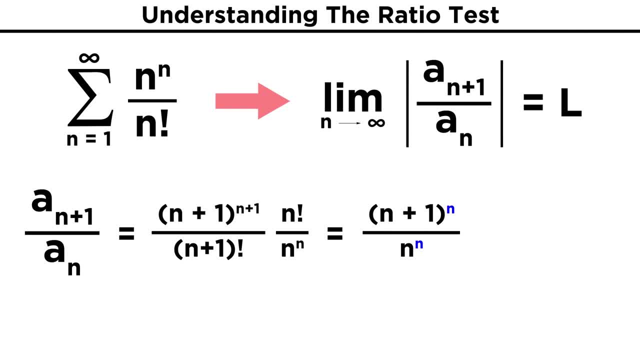 the n. Since these have the same exponent, let's pull it out here to get n plus one over n. all to the n power. We just have to be clever one more time and divide through by n to get one plus one over. 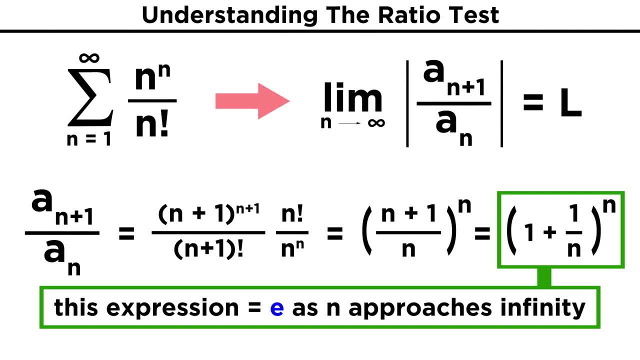 n and recognize that this is actually equivalent to e. Easy to see huh, described earlier in the series E, or Euler's number is around 2.72, and that is greater than one. so according to the ratio test, this series must be divergent.